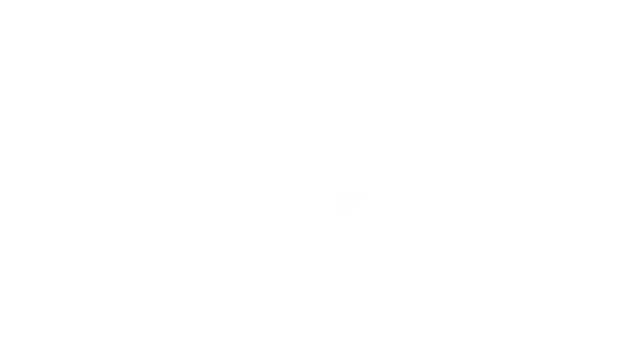 Throughout most of human history, humans' primary source of energy was wood, which we burned to keep us warm and cook our food. However, over the past 200 years or so, this has changed dramatically, Although many people in developing countries still rely on wood. 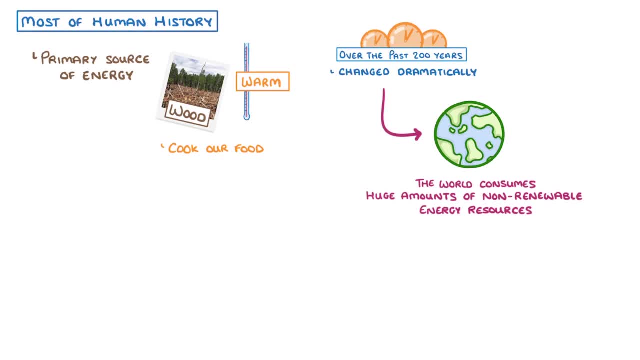 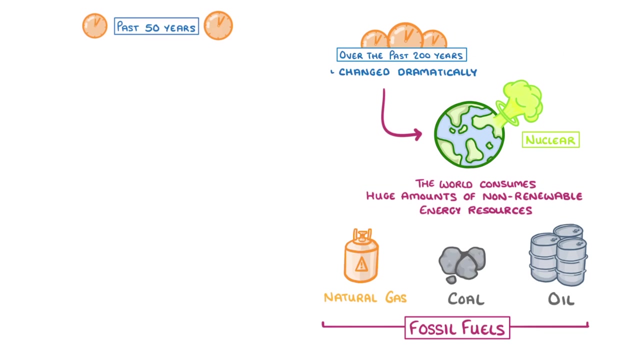 as their primary form of energy. the rest of the world consumes huge amounts of non-renewable energy resources like coal, oil and natural gas, which we refer to as fossil fuels and nuclear energy. In the past 50 years, though, there has also been a massive rise in the 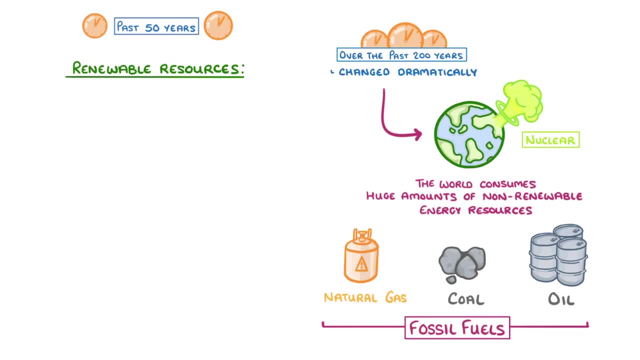 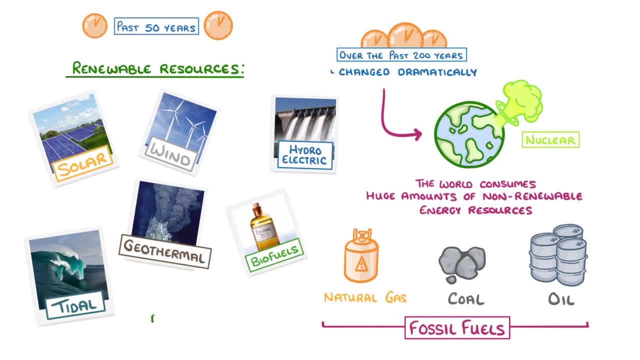 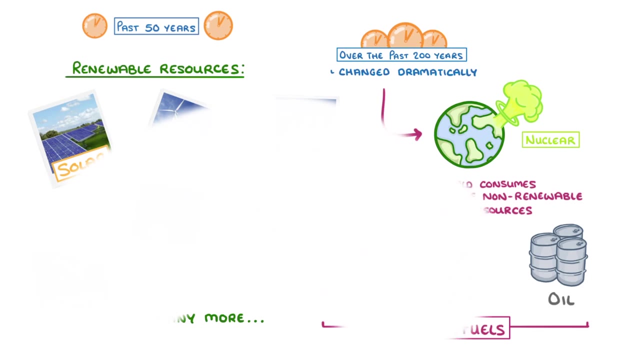 use of a new generation of renewable resources, including solar, wind, hydroelectric, geothermal, biofuels, tidal and many more, And we'll take a closer look at each of these types in other videos. Now the first thing we need to look at is what all of this energy is actually used for. 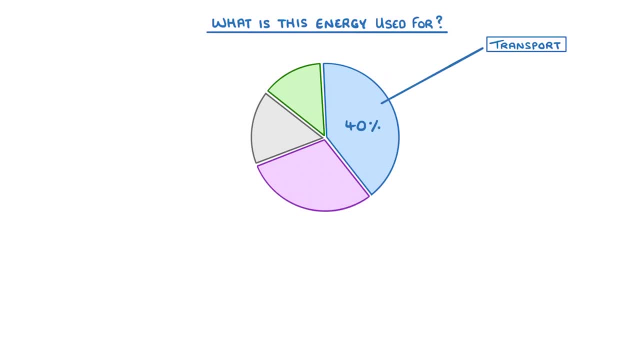 Here in the UK, most of our energy goes on either transport or domestic uses. Transport refers to things like cars, trains, planes and ships, to name just a few, and primarily relies on petrol and diesel in the case of road vehicles and kerosene for planes, which 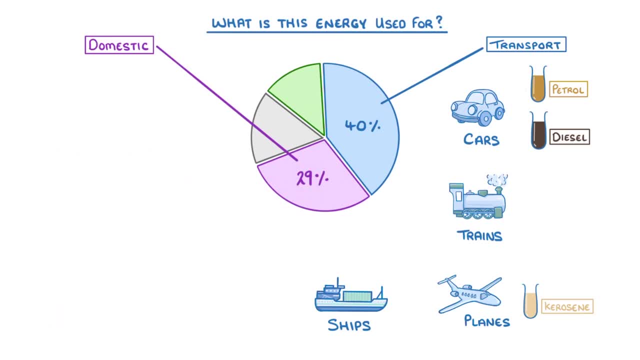 are all created by the use of kerosene. Do you know that all of this energy is created from oil and thus fossil fuels? Traditionally, trains were powered by coal, which helped drive the industrial revolution after coal was found in Britain, but now most trains are powered by electricity. More recently, 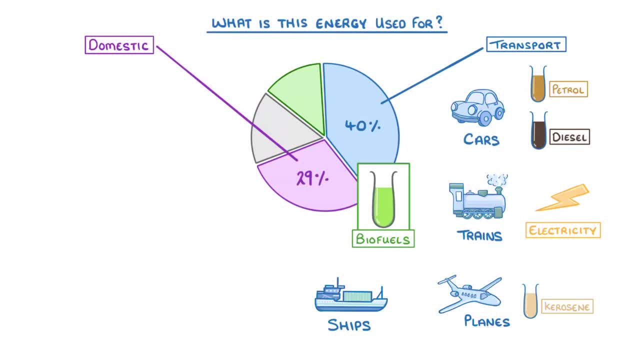 there has been an increase in the use of biofuels, which are created from renewable sources like plants, and also an increase in the use of electric cars. Domestic uses, on the other hand, refers to household things such as heat, water and electricity, And there are 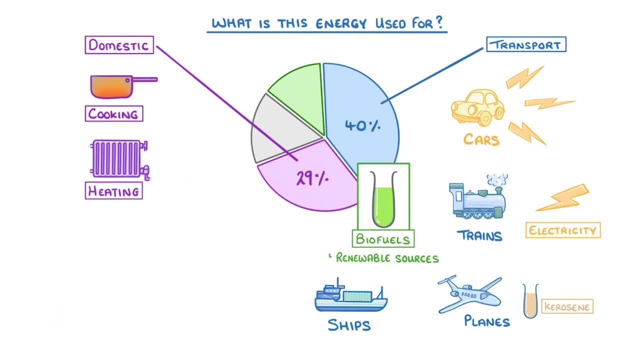 two major sources of power that lead to this. One is that the ability to use the next generation, which is the cost of the energy that is being consumed by the energy industry, has been a significant. things like cooking and heating. For heating, our main source of energy is natural gas.